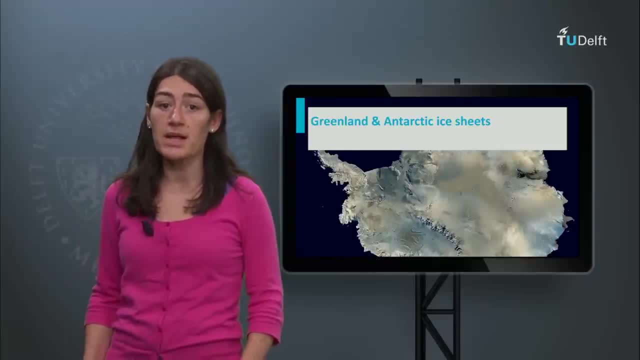 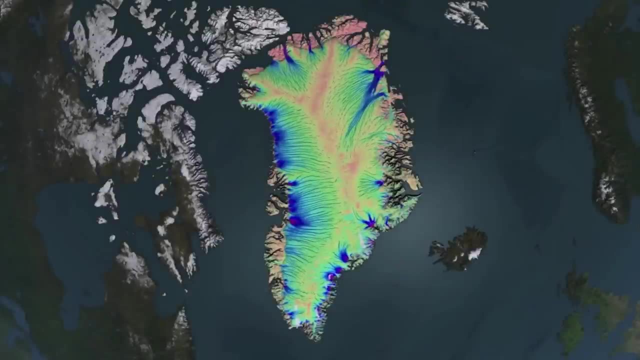 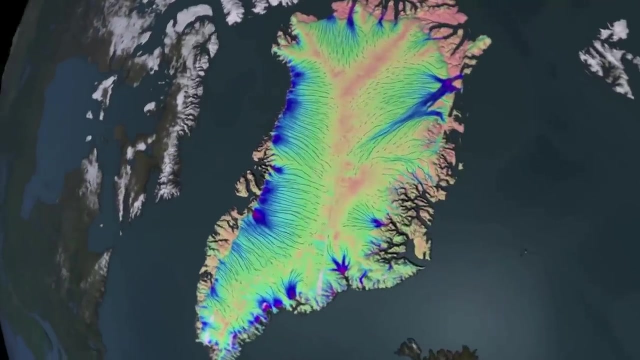 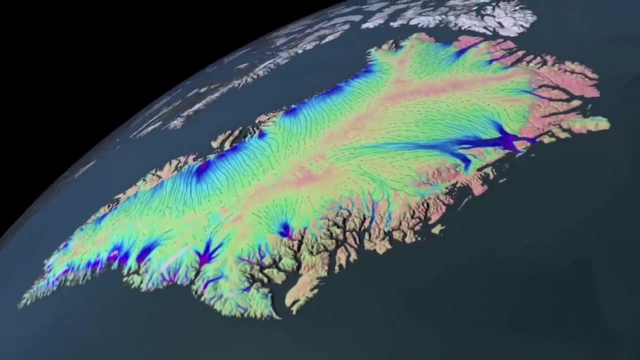 The continental size. ice sheets of Greenland and Antarctica have 7 and 56 meters respectively. Ice is a viscous fluid that moves due to gravity. For grounded ice, velocities increase from the bottom layers to the surface. At the lower boundary with the bedrock, ice velocities are null in the absence of liquid water or sediments. 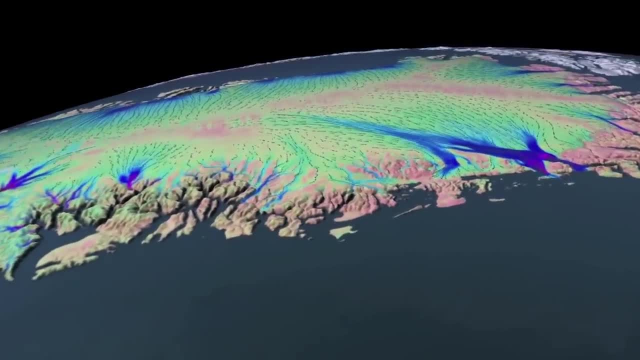 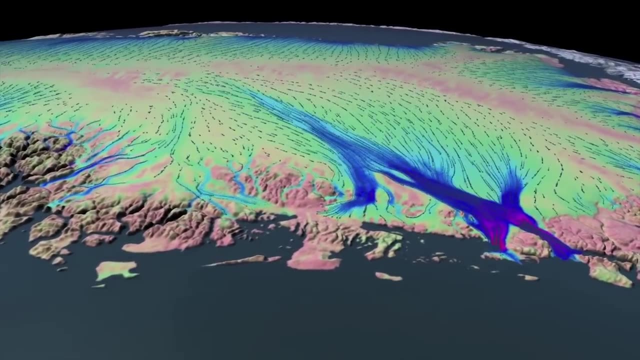 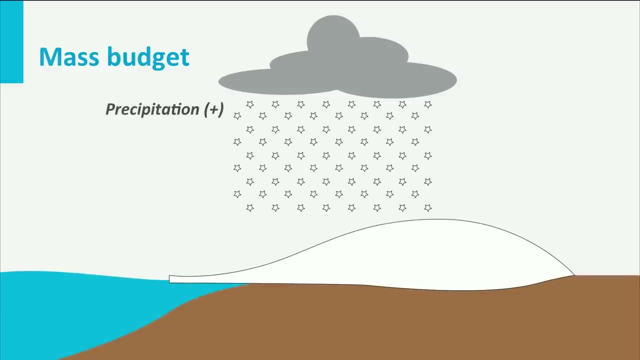 In the places with a sliding or high slope, velocities are high In the ice sheets. surface velocities range from some meters per year in the interior to several hundred at the margins. Glaciers gain mass through snowfall At the surface. they lose mass due to surface melt and runoff and sublimation. 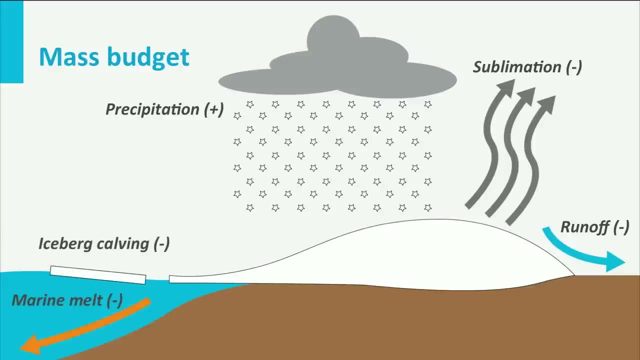 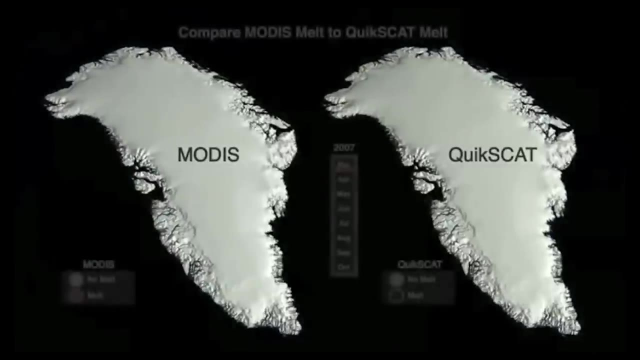 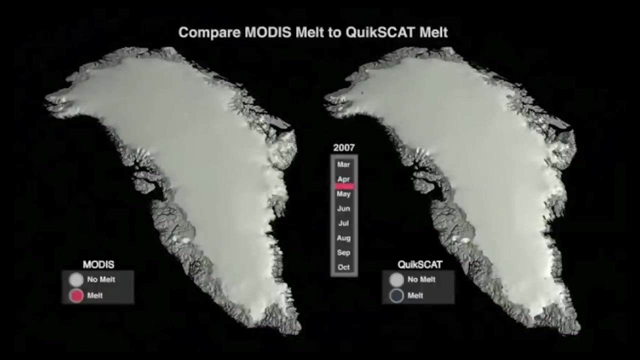 In the places where land ice reaches the ocean, it melts from ocean heat and produces icebergs. Increased ice flow results in higher discharge to the ocean Due to its warmer climate. Greenland has surface melt, Antarctica almost none. Almost all glaciers and ice caps have surface melt, except some high altitude glaciers like Kilimanjaro, which loses mass through sublimation. 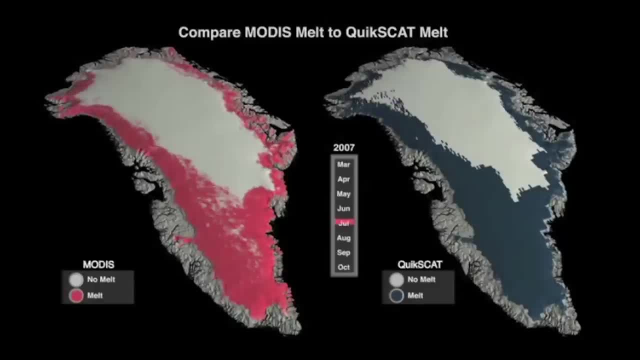 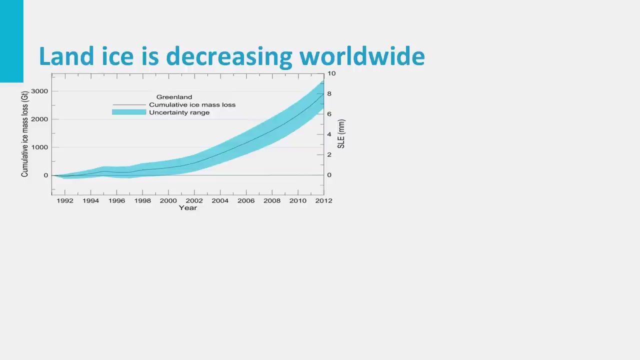 Surface melt occurs during spring and summer at low elevations. An important fraction of melt water usually refluxes within the snowpack and does not contribute to runoff. When an ice body is in equilibrium, the gains from accumulation are balanced by the losses from ice discharge, runoff and sublimation. 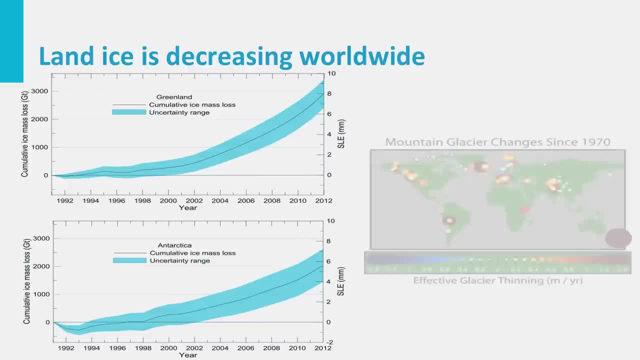 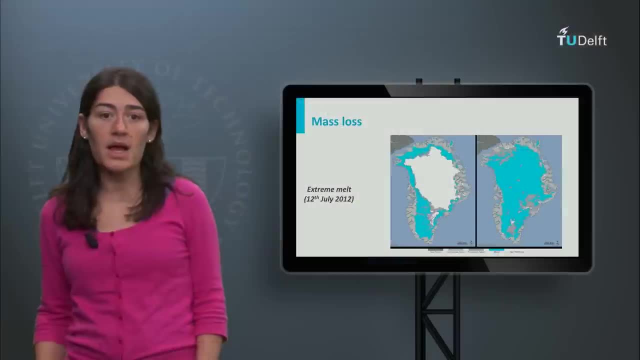 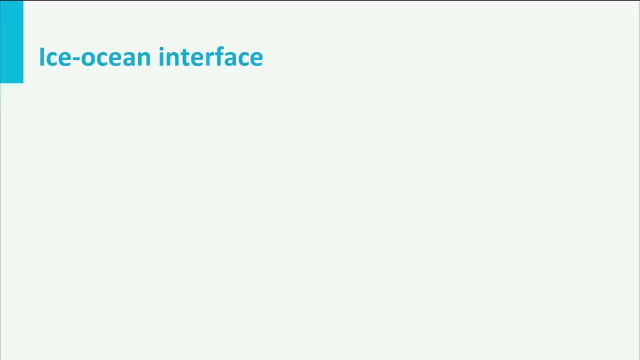 At the moment, most of glaciers and the two ice sheets are losing mass. The Greenland ice sheet is losing mass due to similar contributions of increased melt and higher velocities. The Antarctic ice sheet is losing mass only due to higher velocities. In an ice sheet, ice flows from the dry, cold interiors to the margins. 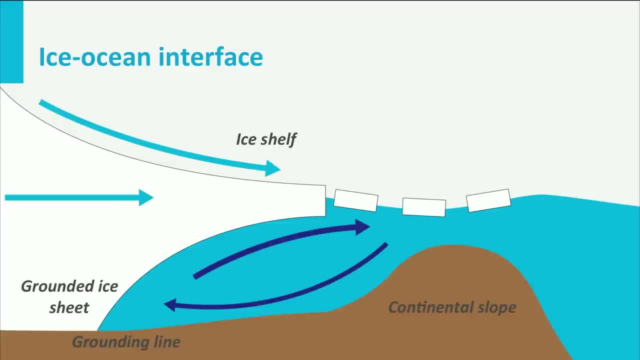 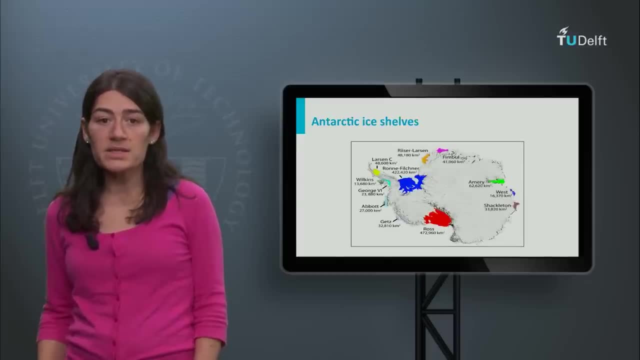 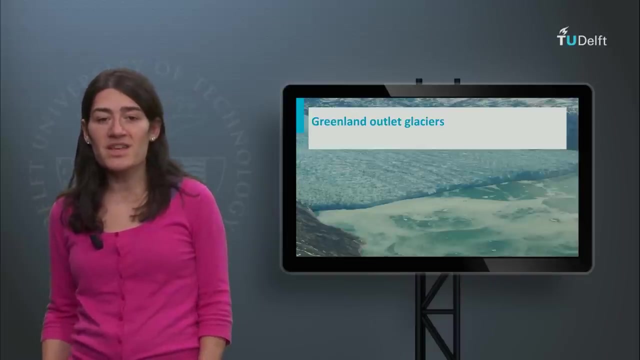 When it reaches the ocean, it may float or move on contact with the submarine bedrock. In Antarctica, most of marginal ice floats in the form of ice shelves, some of them with an area equal to Germany. In Greenland, most of ice is discharged through glaciers of a few kilometres width that do not have a floating tank.